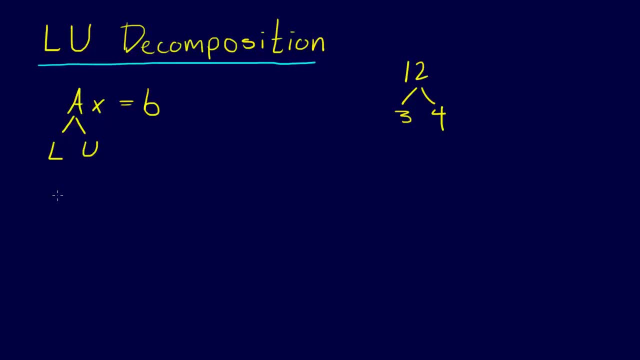 Where L- you'll recall perhaps from our discussion on matrices- where L is a lower triangular matrix, meaning again that we have entries, non-zero, entries below the diagonal and on the diagonal. Okay, so if that's the case, we're going to do that. 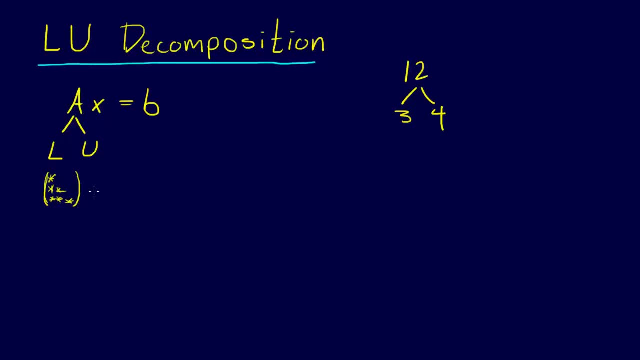 Okay, so if that's the case, we're going to do that. That's a 3 by 3,, for example. That would be, our L would look something like that and our U is going to have again along the diagonal, and then it'll have non-zero entries here. 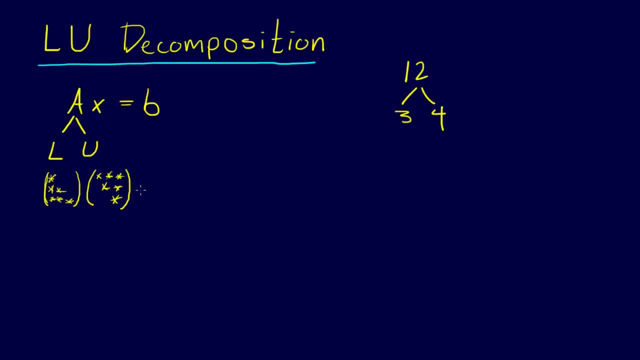 So this is the sort of structure. LU is a decomposition that we can do on A. Okay, so with LU decomposition, step one. Step one is: step one is: decompose A into LU. okay, Step two: compute. I'll just put figure out. 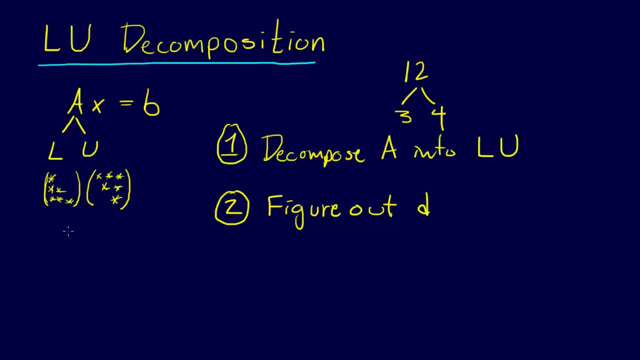 Step two, compute. I'll just put figure out D and let me explain that. So we go from this matrix: AX equals B, and if we want to rewrite this, we could say: AX minus B equals zero. and then we go. what we do is we factor an L out of A, but we can also factor an L out of B. 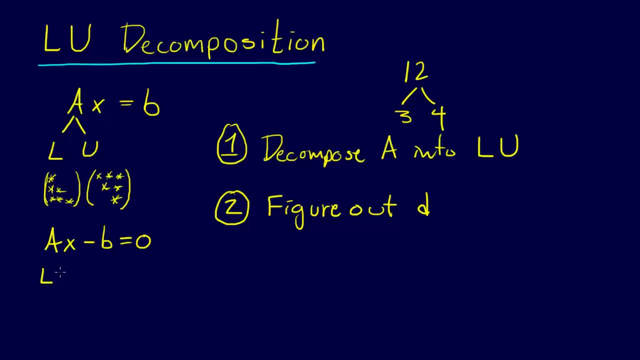 And so we can say L Um U, and I'm going to put a parenthesis: LUX minus LB, LB, and I'm going to call that: D minus D equals zero. That's because that's just L times U is A and L times D is B, and so let me just I can write that as well. 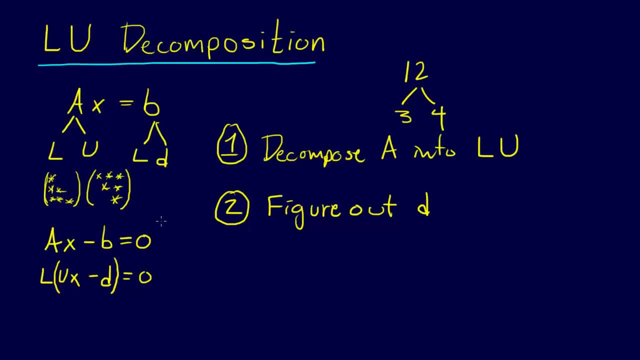 L, Uh, D, okay, Uh, matrix vector product, and we get B, Okay. so number two is figure out D, And you have to realize when we do that then we have what we have for D is the. the equation L, D equals B. 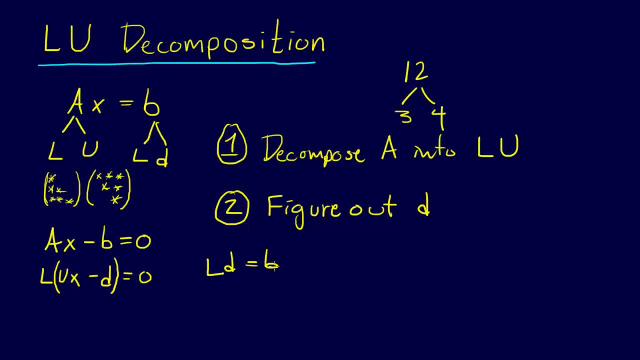 And uh recall this is: this is a simple equation to solve relatively. We have B, uh, we have L, and L has this nice lower triangular structure, And so we can figure out D by doing uh forward substitution. 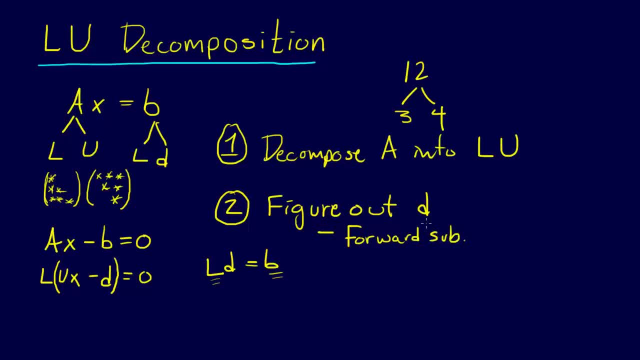 Forward substitution Because, uh, we just have, um, well, L, L, D equals B, so so the first uh D entry uh is anyway. So it's, this is relatively easy to solve because we just do forward substitution. 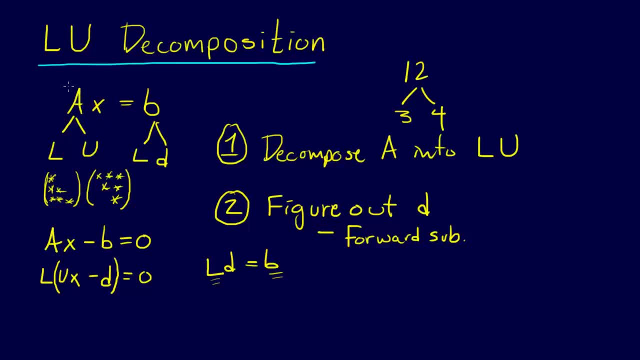 We have this triangular matrix. It's: it's a similar problem: AX equals B. Right, We have a matrix, we have a vector and we have a vector. we have a matrix, a vector and a vector, and we're trying to figure out this unknown vector. 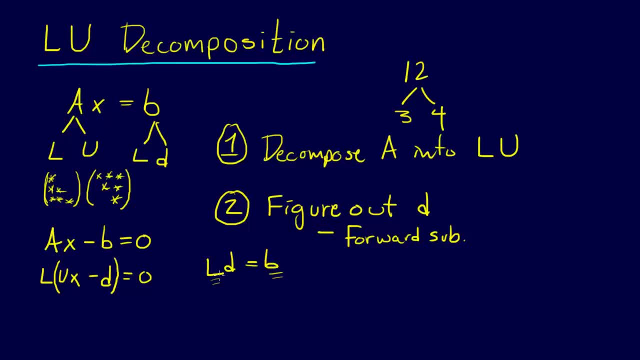 But this is easy to do, uh, uh, because this is a triangular structure, so we can just do: uh, forward substitution. Now step three: Okay, so we've done that, so let we do that. so we've got D, uh, and then step three is solve, uh, solve for X. 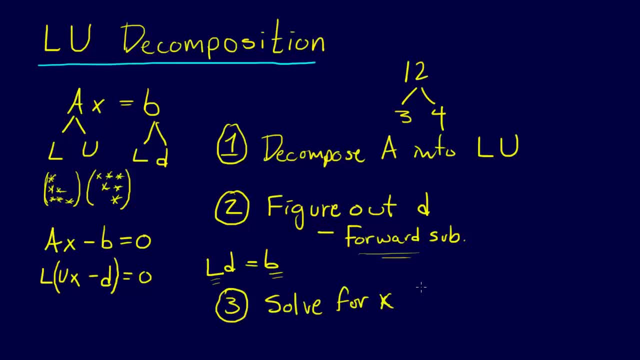 We solve for X, and that is what we're. the equation we're solving is um see UX minus D equals zero, and so U. this also means because we could, we could, we could get rid of this L, so this also means UX. uh, excuse me, that's again undo on that. 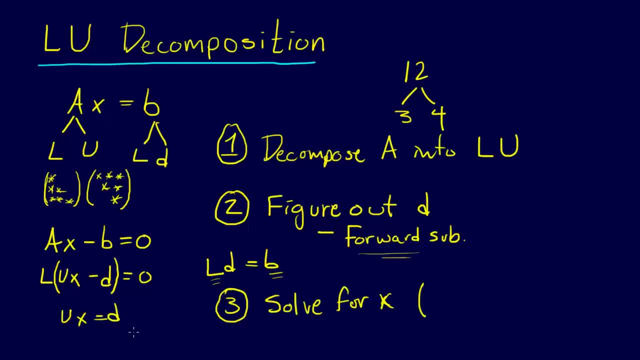 So U X equals D. Okay, so we can solve that equation. and uh, so uh U X equals D, and we've got D from the previous step and we've solved. we've solved that equation and that again is easy, because that is just uh back substitution. 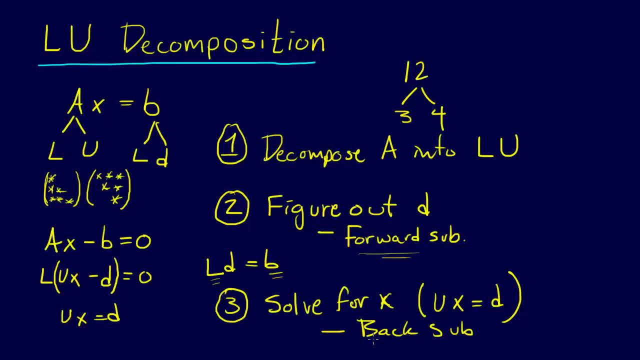 Because of the nice triangular structure of U. Okay, so there we have LU decomposition. This is what you do: You decompose. You decompose A into L and U. We got that. Uh, we figure out D, because LD equals B.